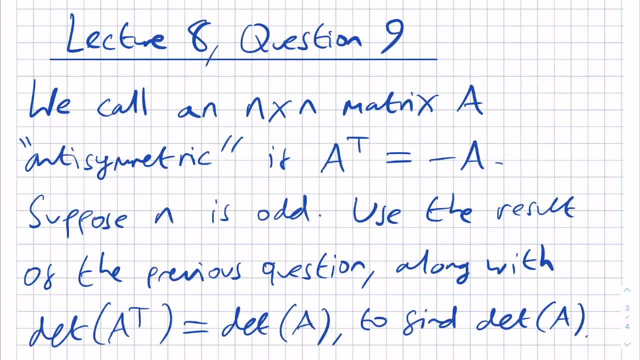 Hi everyone, this is Maths4Uni. This is the worked solution to questions 9 and 10 from Lecture 8.. If you enjoy this content, then please consider liking and subscribing, as well as checking out our full Udemy course, of which the link is in the description. 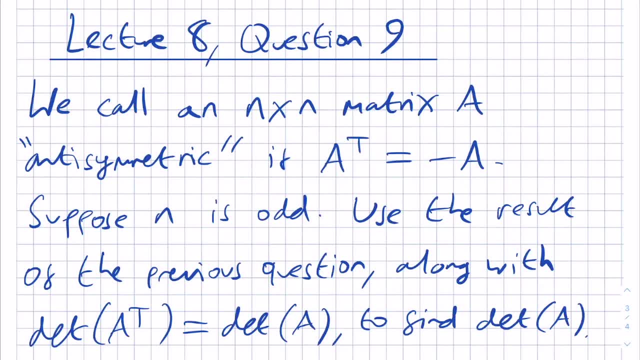 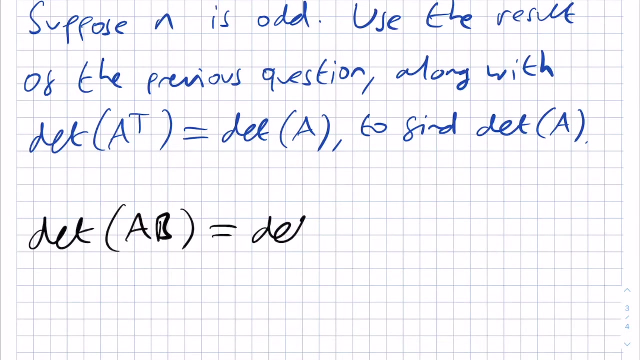 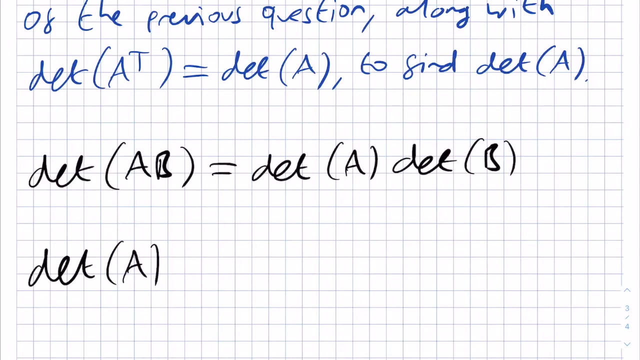 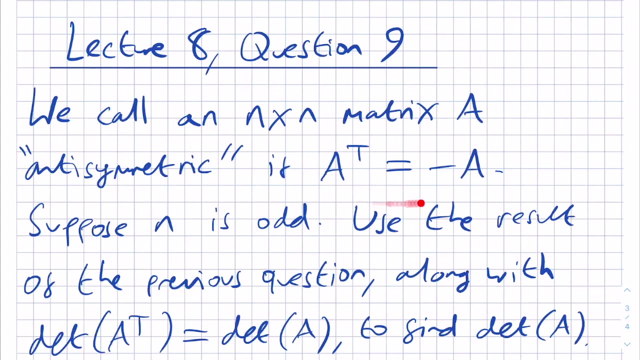 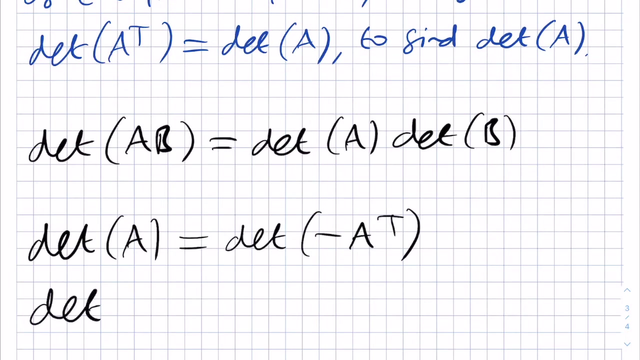 The question says: The result of the previous question is the one that we considered in the previous question. We want to find the determinant of A as part of this question. We note that At this point we want to use that debt of A. transpose is always equal to debt of A. 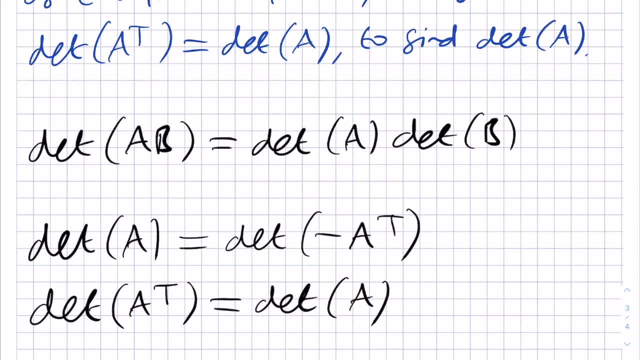 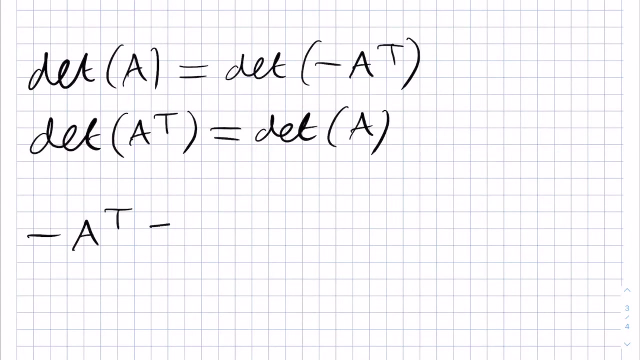 However, we should be careful because of this problem. We need to split up our debt of minus A transpose using the product of the determinant's result. Notice that minus A transpose is equal to minus the identity matrix multiplied by A transpose, where I is the n by n identity matrix. 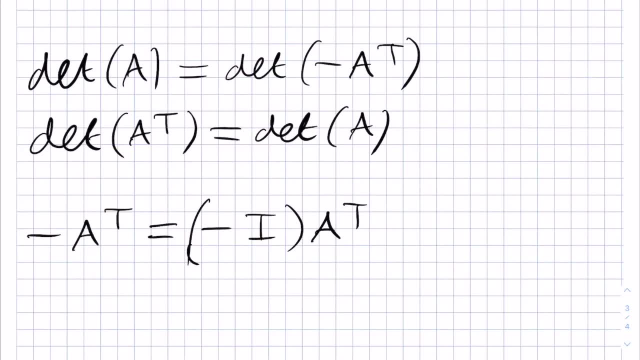 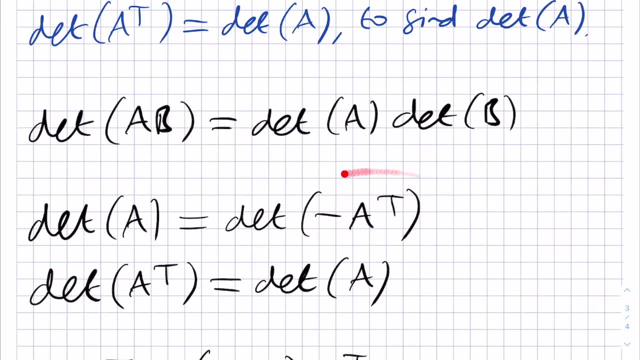 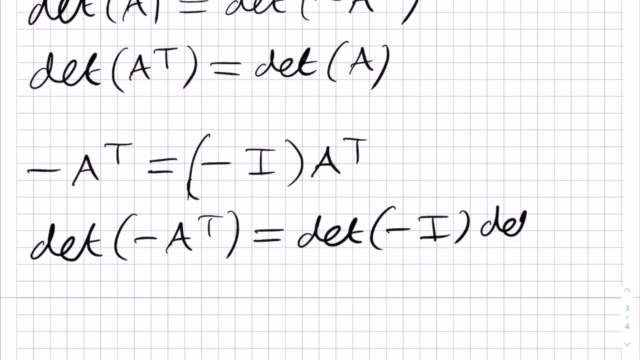 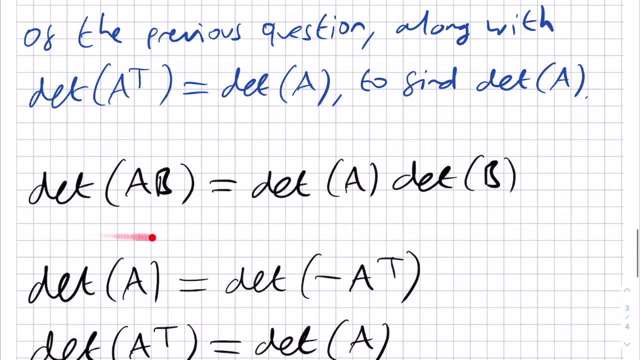 Hence, from the result of the product of determinants, we have that debt of minus A transpose, which we're looking at here, from debt A is equal to debt of minus. I times debt of A transpose by using this result here and this result here. 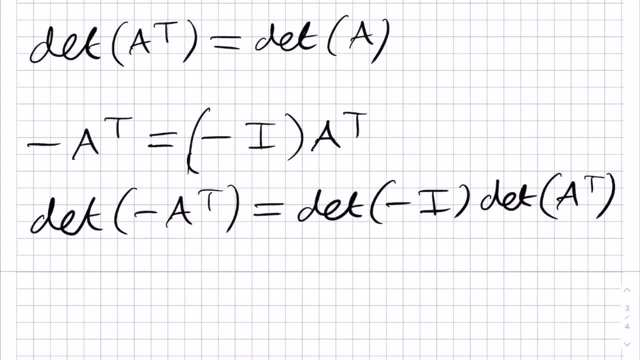 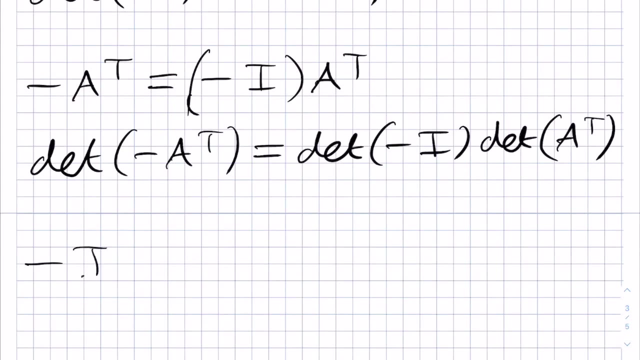 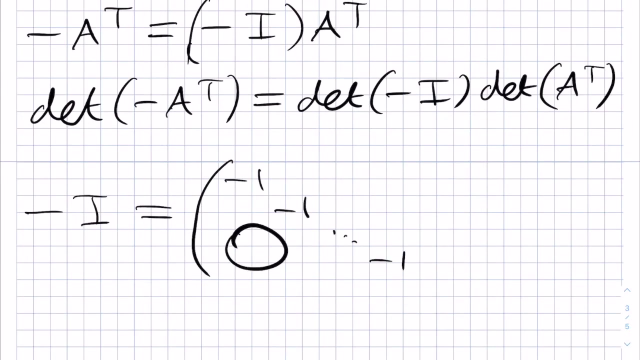 Then we should next calculate, calculate the depth of minus i, since it's an explicit matrix that we can consider, whereas a is some general anti-symmetric matrix. Minus i is the matrix that has minus 1 in each of its diagonal elements, with every other element being a0, which we can write like this There: 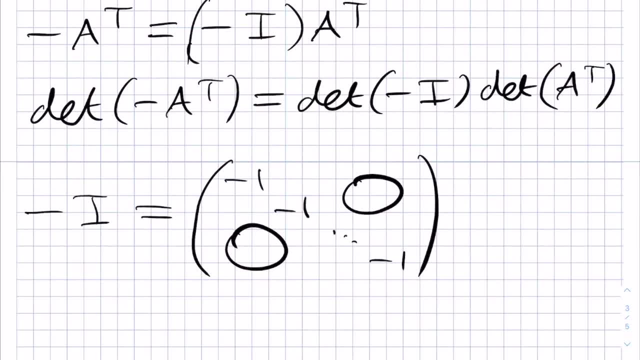 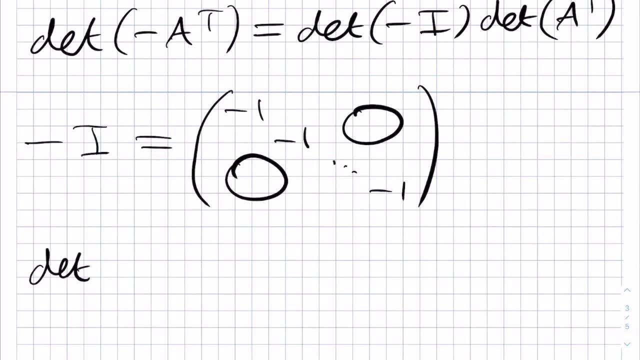 are n minus 1s here, because it is an n by n identity matrix and therefore the determinant of minus i is equal to minus 1 to the power of n. This we can show inductively, but we won't do so. 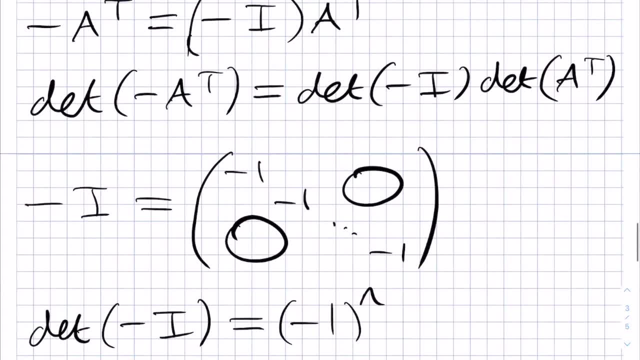 formally here, because you can imagine working out the determinant of minus i as a 0. We can do this by doing minus 1 times the determinant of this matrix here, where we get rid of this column and this row, but this matrix here will be the n minus 1 by n minus. 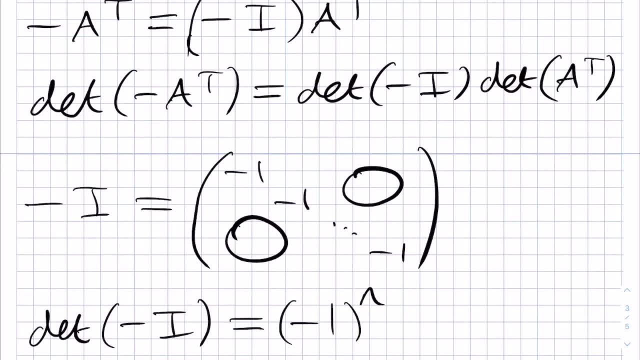 1 identity matrix. Then we go down continually inductively using this and either way we end up by picking up n factors. Now we were told in the question that n is odd and so minus 1 to the n is minus 1.. 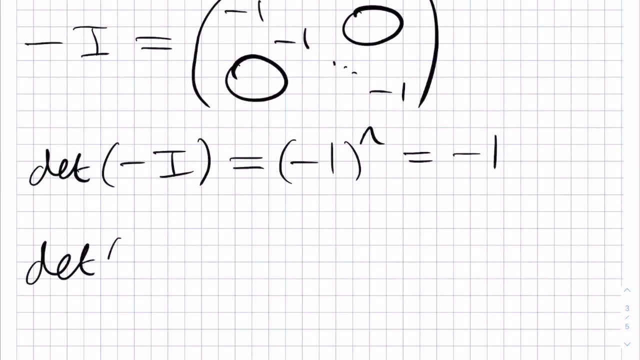 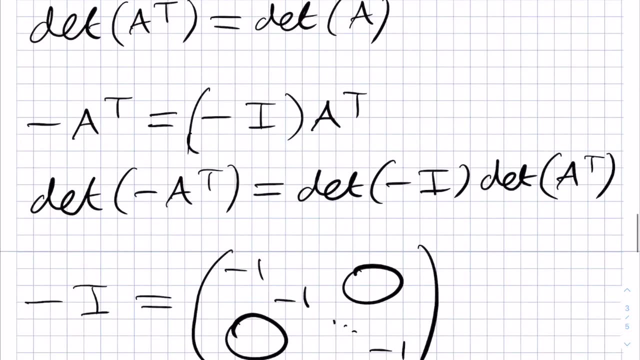 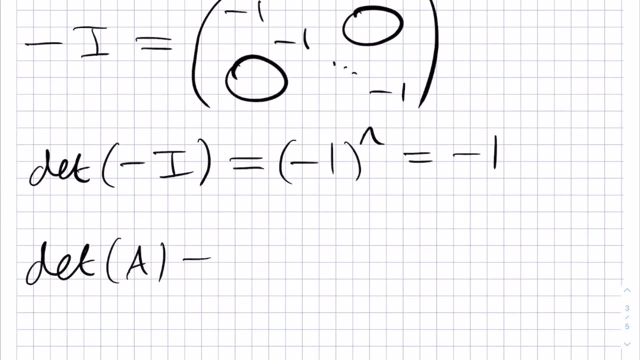 This tells us that the determinant of a that we want to calculate is equal to this thing here, which is equal to: as we showed this thing here Then we have, since this is minus 1, we have minus debt of a transpose, but we were told that debt of a transpose is equal. 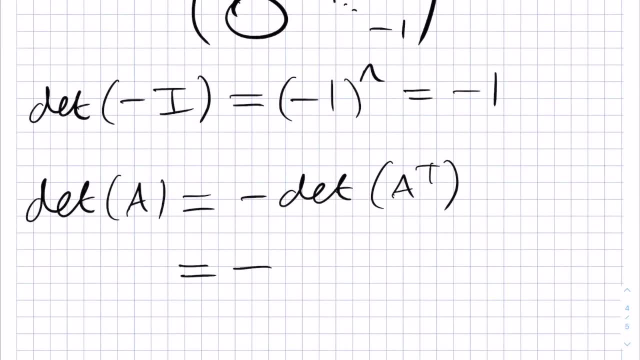 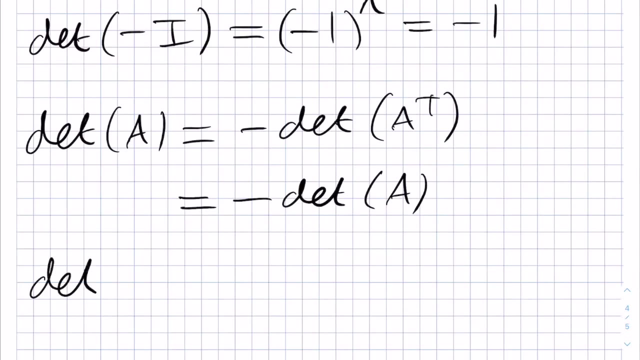 to the determinant of a. so this is minus debt of a. The only number such that you get it being equal to minus itself is 0, and therefore the determinant of a must be 0.. Now to finish off with this question, at least if we weren't careful with the minus. 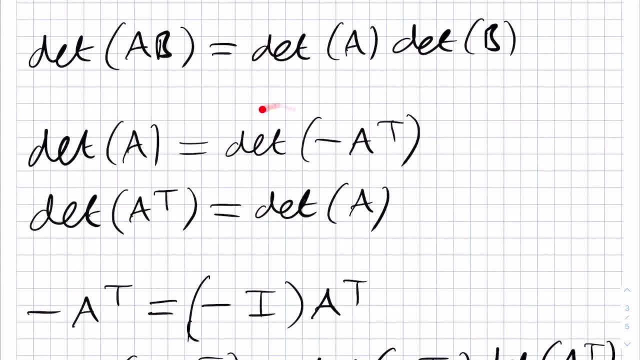 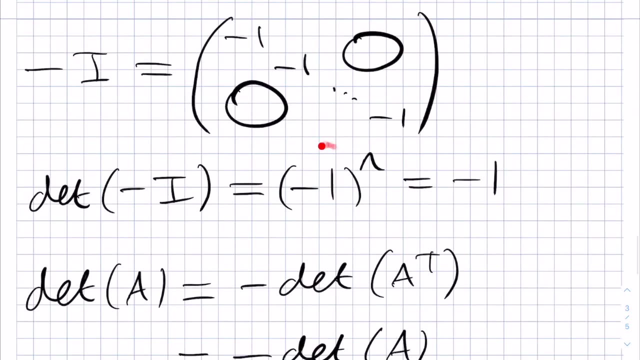 sign in this determinant of minus a transpose, then we would have ignored a small subtlety. If n is even, then this result that we've shown here is not true. How can a sum of everything considered an even number be even? How can a sum of everything considered an even number be even? How can a sum of everything? 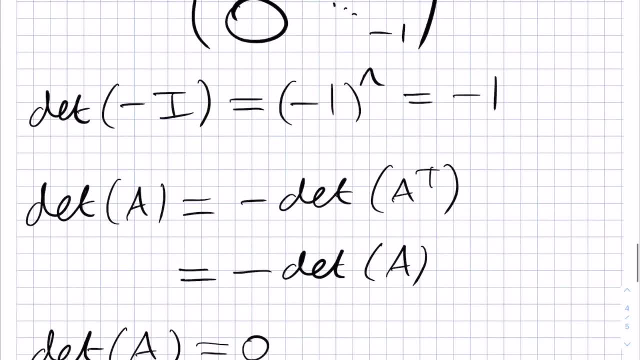 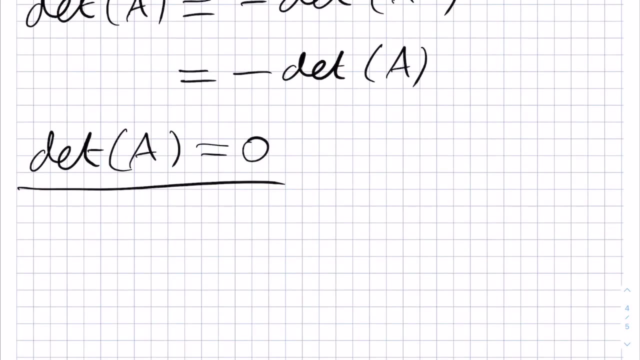 1 to the n is plus 1, and so we'd get debt A equals debt A, which is fine. As a result, we cannot get debt A equals 0, like we did above. However, if we were to wrongly just proceed ahead and assume that, in full generality, debt of minus A transpose is equal to minus, 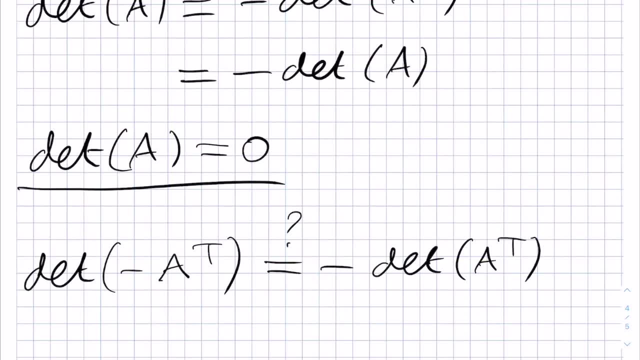 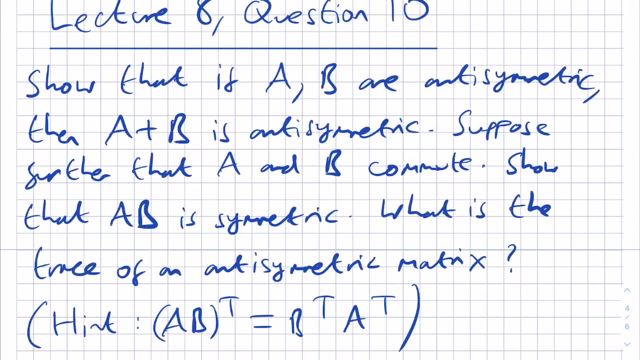 debt of A transpose, ie pulling out the minus sign, then we would get the wrong conclusion for the case that n is even because this result here only works when n is odd, as we showed. Next let's discuss question 10.. The question says: show that if A and B are: 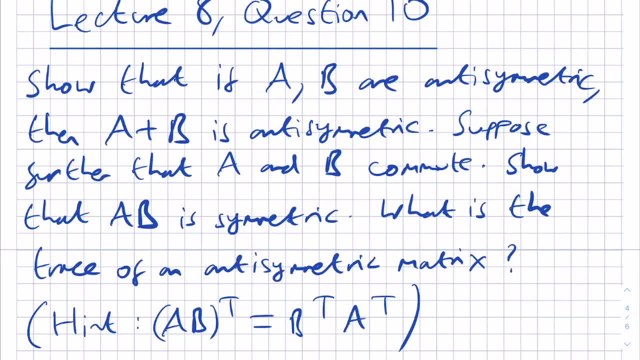 anti-symmetric, then A plus B equals 0.. A plus B is also anti-symmetric. Suppose further that A and B commute. Show that AB is symmetric. Finally, it asks: what is the trace of an anti-symmetric matrix? And there: 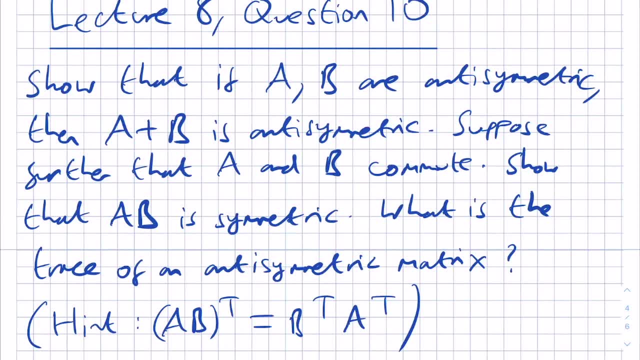 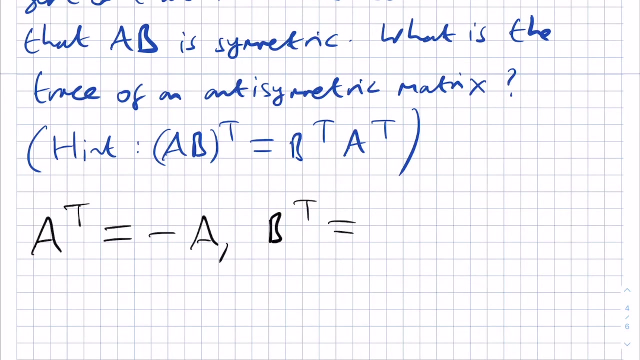 is a hint for this question- that AB all transpose is B transpose, A transpose, ie we reverse the order. Firstly, if we assume, as we are told to, that A and B are anti-symmetric, then we have that A transpose is equal to minus A and that B transpose is equal to minus B. Then 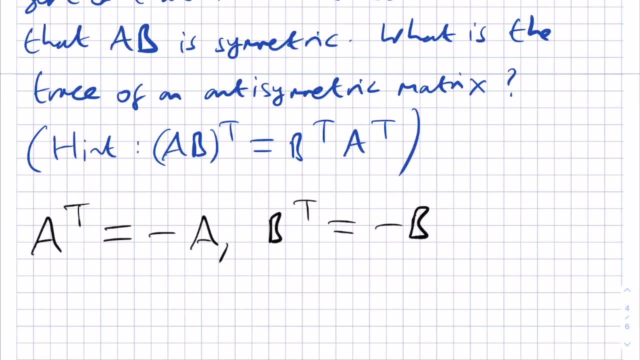 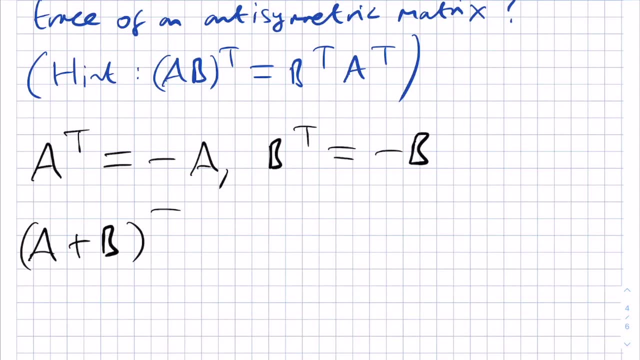 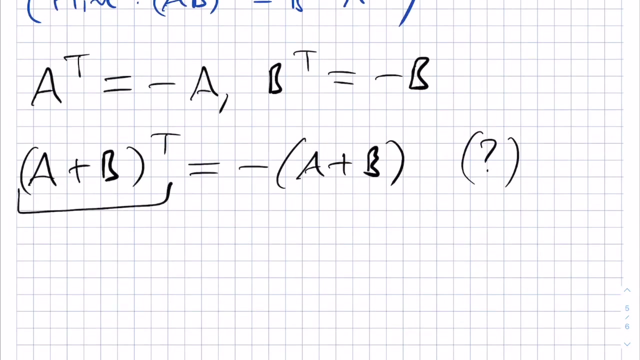 we want to show that A plus B is anti-symmetric. This means that we want to show that A plus B- all transpose is equal to minus B. If we look at the left-hand side, then we first have that A plus B- all transpose is. 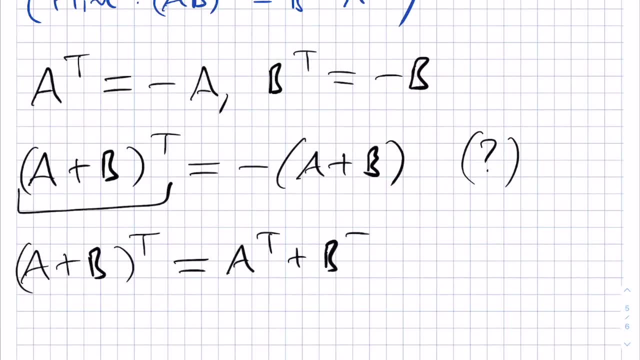 equal to A transpose plus B transpose, And this is just by separating out the transpose over addition, which should be 5.. So if we look at the left-hand side, then we first have that A plus B. all transpose is fairly clear. If it's not, then have a go at putting in some example matrices to convince. 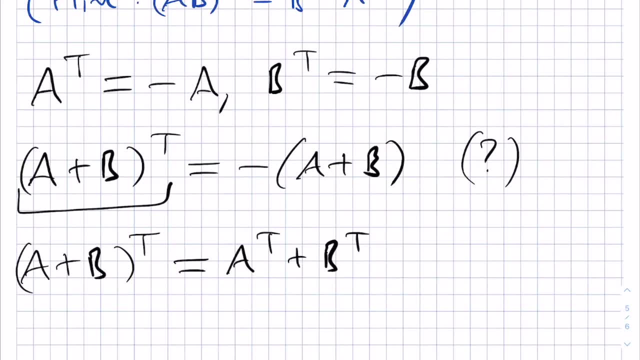 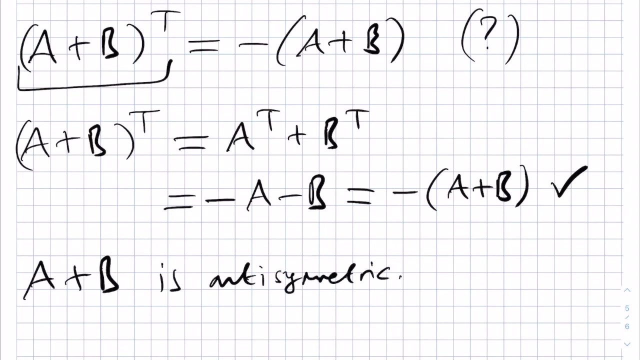 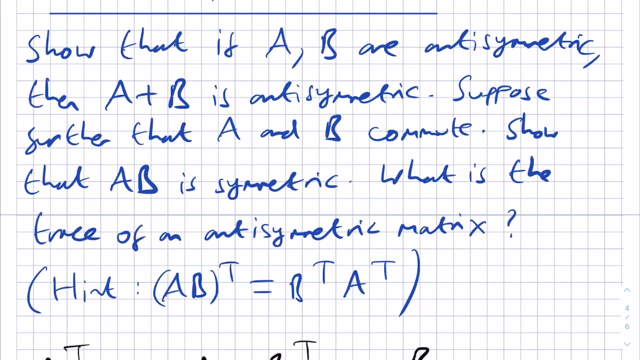 yourself. Then, because A transpose is minus A and B transpose is minus B, we get minus A minus B here, which, by factorising, is minus A plus B. Indeed, therefore, A plus B is anti-symmetric. Next, we want to show that A times B is symmetric, given also that A and B commute. ie, we want 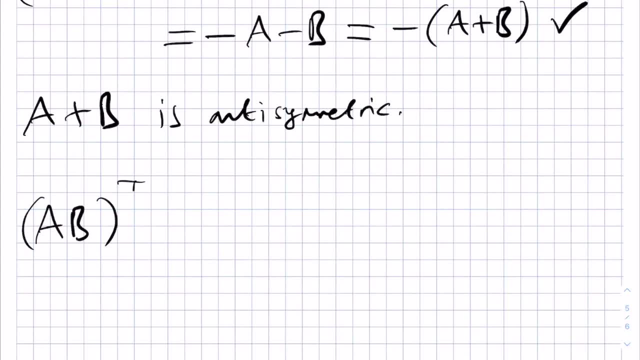 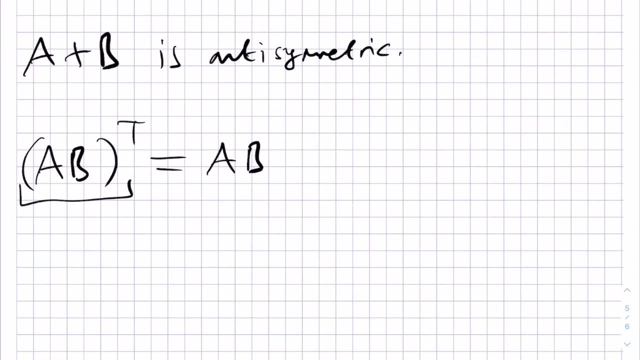 to show that the matrix A times B transpose is equal to A times B, just like anti-symmetry, but without the minus sign. Firstly, using the hint we have that the left-hand side is equal to B transpose times B A transpose. Then we can use the anti-symmetry of A and 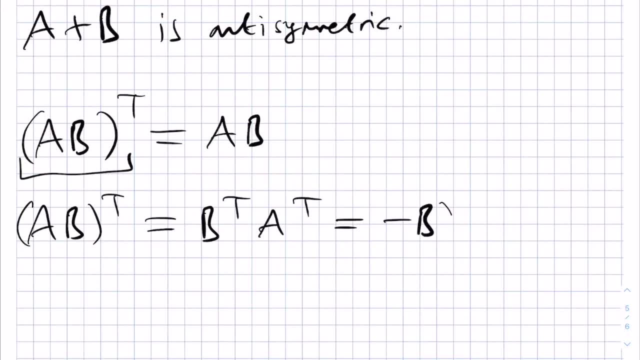 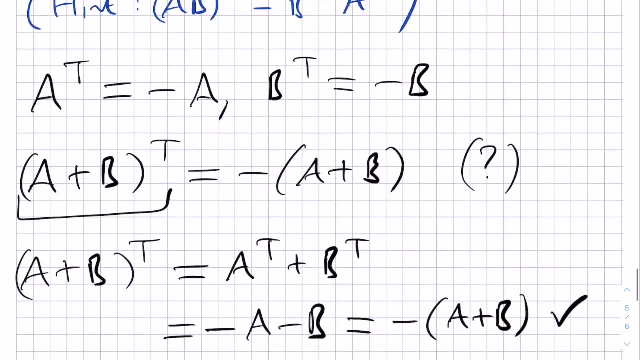 B. Then we have minus B for B- transpose and minus A for A- transpose. The minus signs cancel because there are two of them, and so we get B times A. Then finally, as we were told to assume, we can use that A and B commute, and so the order in which they're. 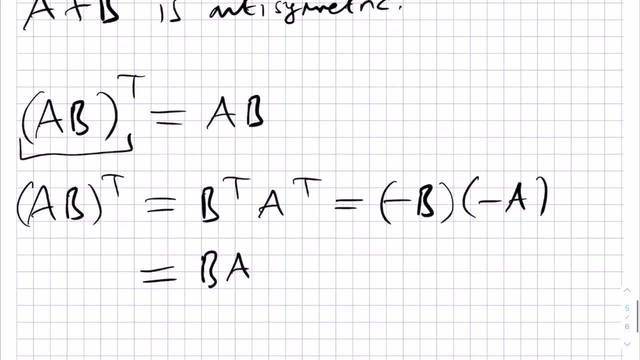 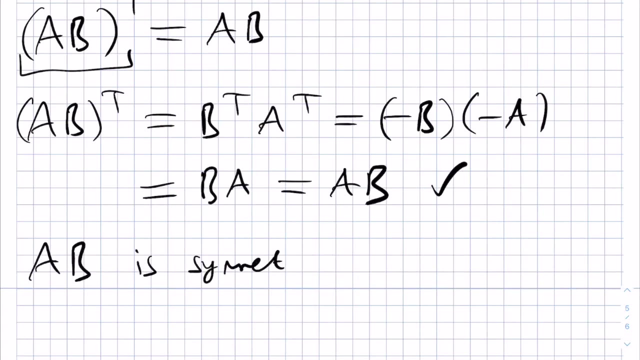 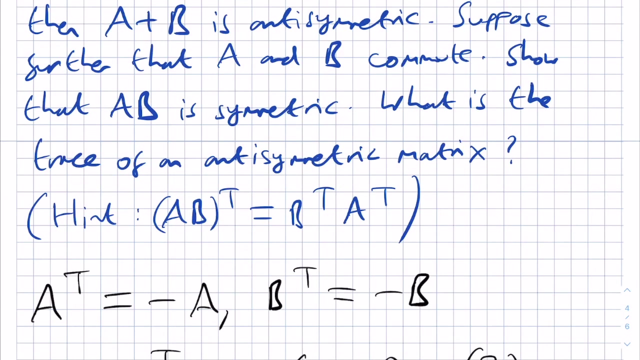 multiplied do not matter. So B times A is the same as A times B. Therefore we have shown via this chain that AB is a symmetric matrix. Lastly, the question asks us about the trace of an anti-symmetric matrix. Recall that the trace is the sum of the diagonal elements of the matrix, and so it only makes sense when.